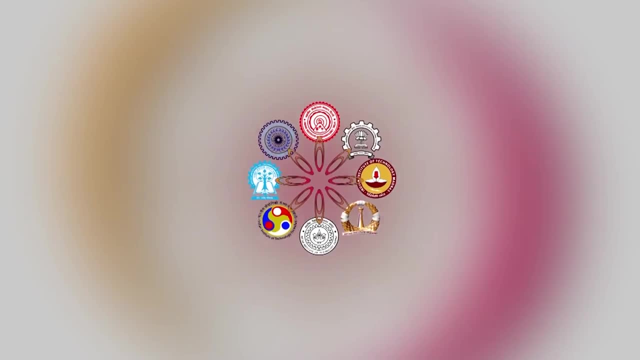 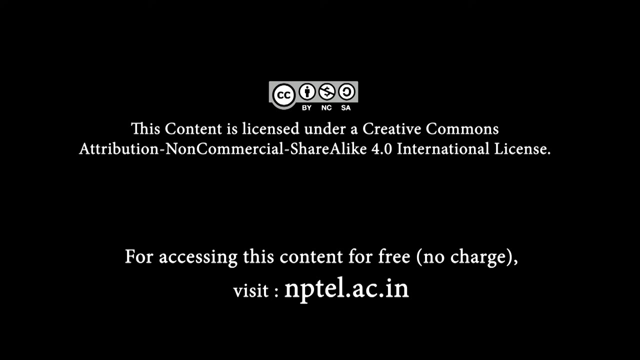 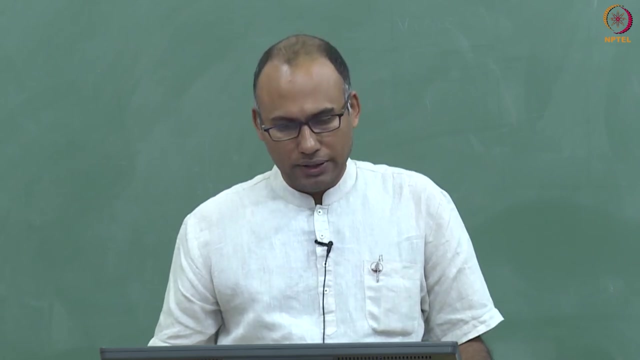 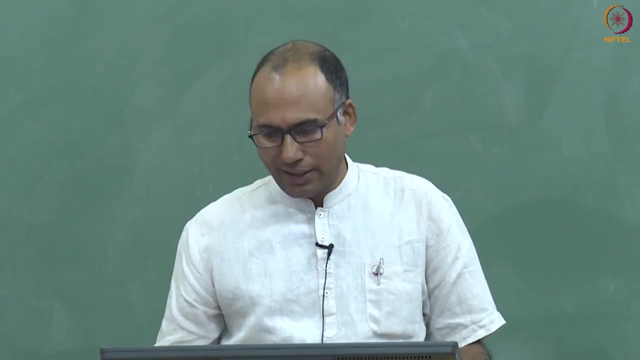 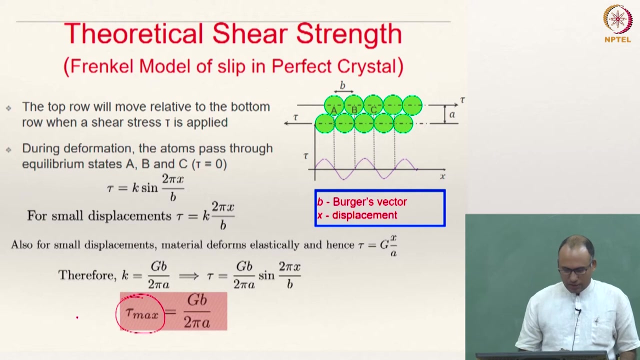 Let us get started. In the last class we have looked at theoretical shear strength. How do we go about calculating the theoretical shear strength of a given material? And then we have seen that the maximum shear stress required to cause slip of one layer of atom, atom plane. 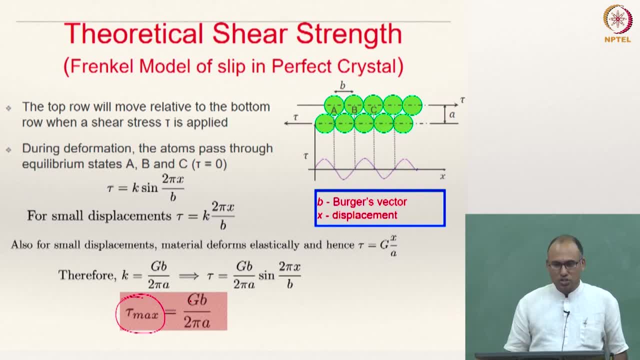 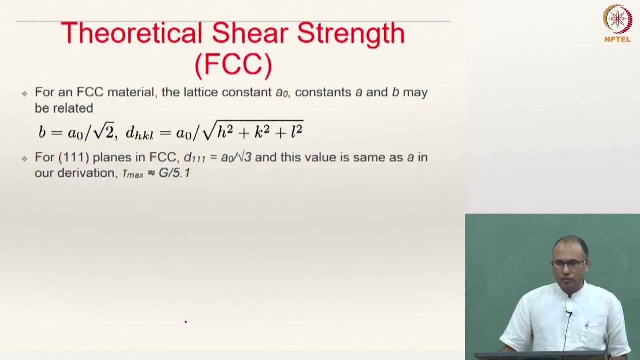 over another plane of atoms is given by the shear modulus times, Burgers vector times- divided by 2 pi a, where a is your inter planar addition. And then so, using this simplified formula, we can actually calculate for any given material what is your tau max right as a function of: 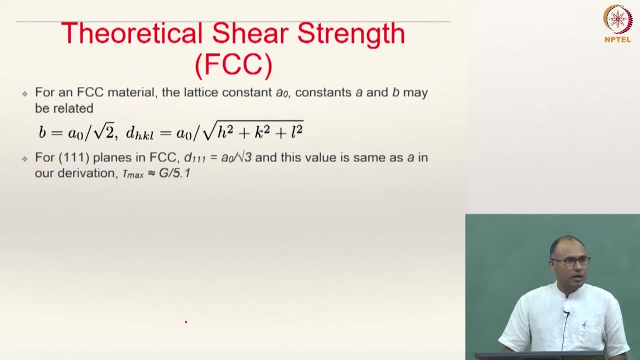 shear modulus if it is an FCC material And if you are talking about shearing flipping over one on one plane, So for one one one planes. you know the inter atomic spacing can be calculated to be a naught by root. 3. 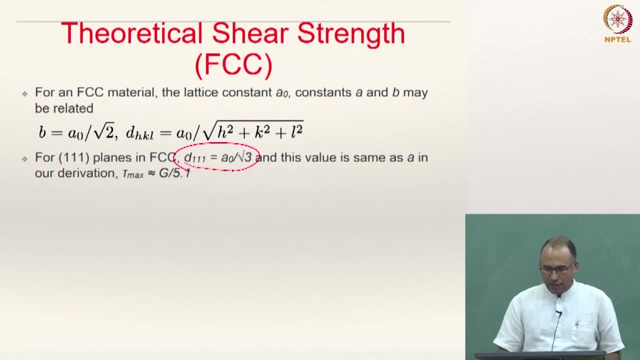 where a naught is your lattice constant right or lattice parameter for the cubic crystal, FCC crystal, And then Then you, we can find out the tau max to be g by 5.1, right one-fifth of the shear modulus. 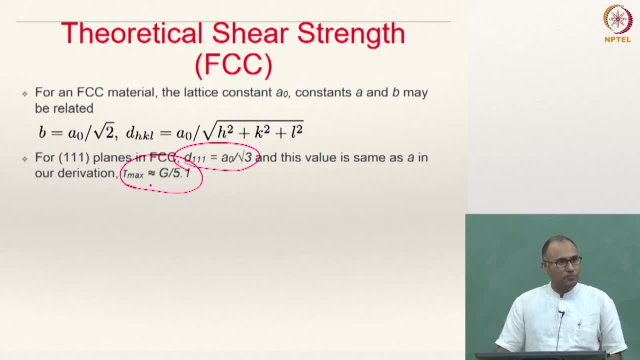 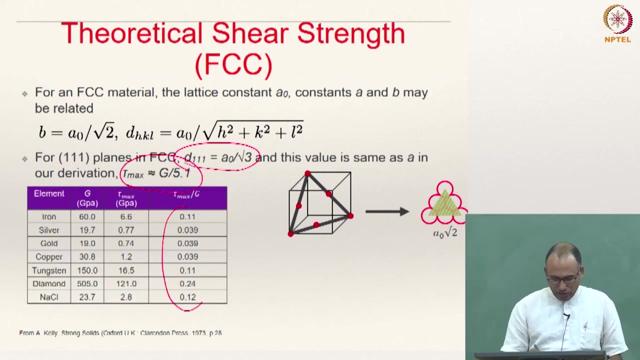 which means the shear modulus and your shear strength or tau max. the shear strength of the material are of the approximately same order of magnitude, right, But the real materials do not have such high value. So you can actually calculate this right. so if you calculate the theoretical values, 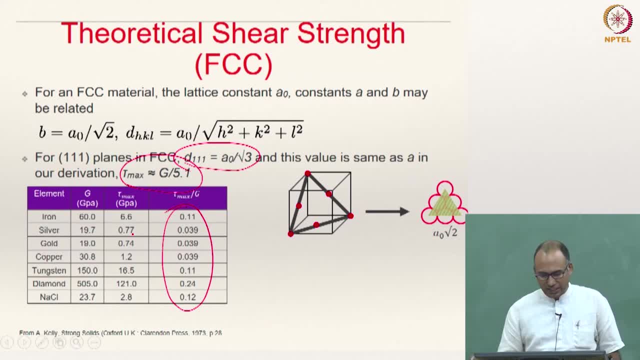 for real materials. so the materials in these idealistic situations it comes out to be, they are at most one order of magnitude different, but otherwise they are all almost same order of magnitude. their value stands out for you right, So you can actually estimate the theoretical values. 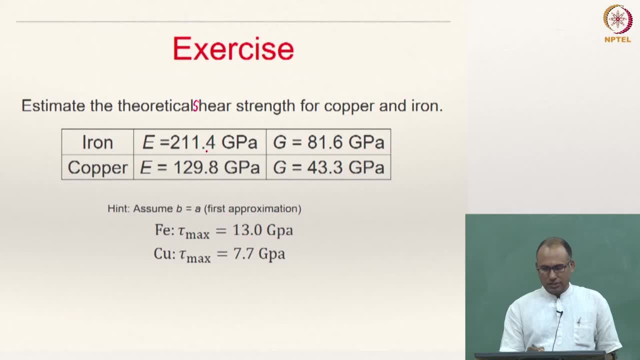 So you can actually calculate the theoretical values. So you can actually calculate the theoretical shear strength of the of copper and iron, given their elastic modulus and their shear modulus. We have just now calculated our tau max is equal to gb divided by 2 pi a, and we can actually 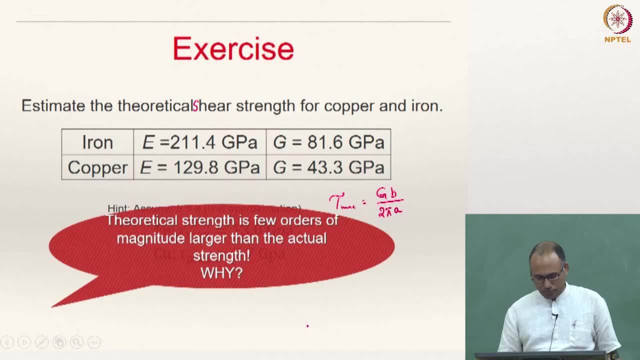 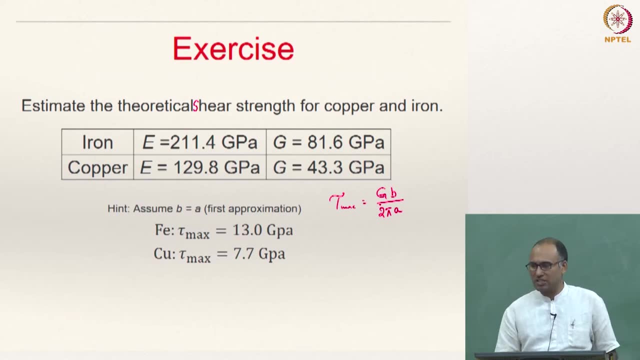 make a reasonable approximation, saying that our intratamic spacing is and interplanar spacing are almost similar. They are not going to be exactly same, but you can actually make a first-hand approximation. If you make such a first-hand approximation, right, then you can calculate your tau max. 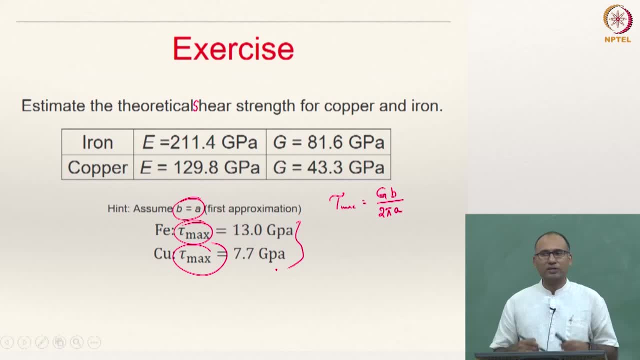 for iron and copper to be in the order of gigapascal, But the real material shear strength is known to be in the order of megapascals. So that is the discrepancy, Why the theoretical shear strength for ideal crystals are not known to be in the order 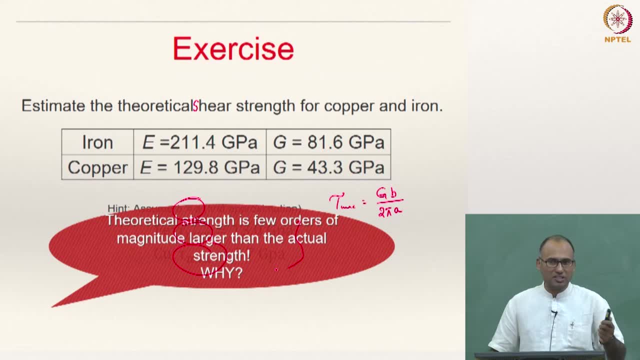 of gigapascals. So that is the discrepancy. Why the theoretical shear strength for ideal crystals are not known to be in the order of gigapascals? Why the theoretical shear strength for ideal crystals are not known to be in the order of gigapascals? 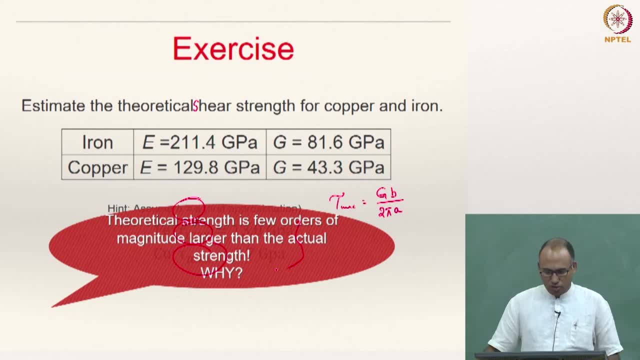 Why the theoretical shear strength for ideal crystals are not known to be in the order of gigapascals. They are just a drop-off of real material. So the real material shear strength is much more much predicted to be much higher, calculated to be much higher, while the real materials do not have such high strengths. 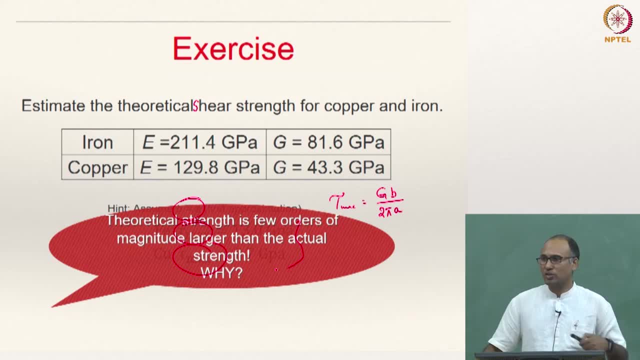 So the origin for these things maybe in the defects. So that is the reason why we probably need to study defects and then try to understand how these defects lead to lower strength to these material. Okay, All right. So so far we are looking at a point: defects. 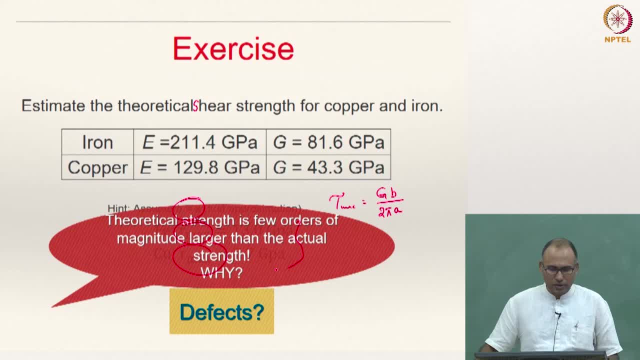 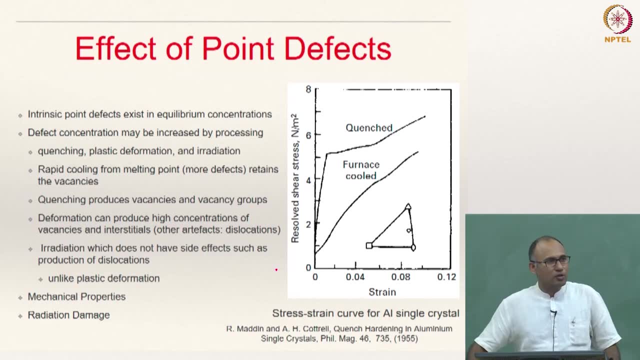 So let us now look at what are the different effects of this material, What are its property, So what are the different effects of these material? So so far we are looking at point defects, So let us now look at what are the different. 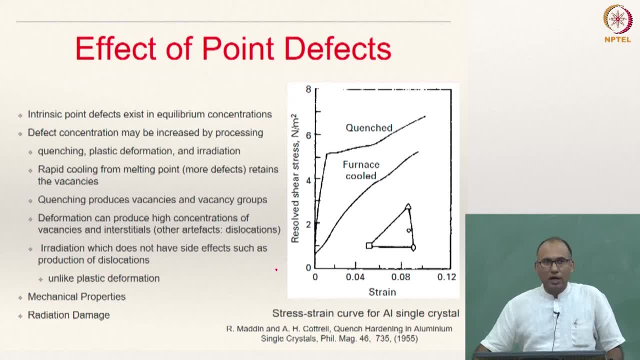 effects of these point defects And we have already discussed in the last class and we have actually derived an expression for equilibrium concentration of vacancies and during that process we have realized that even at room temperature, without actually doing any additional thermal excitation, every material will have some number of vacancies or point defects. 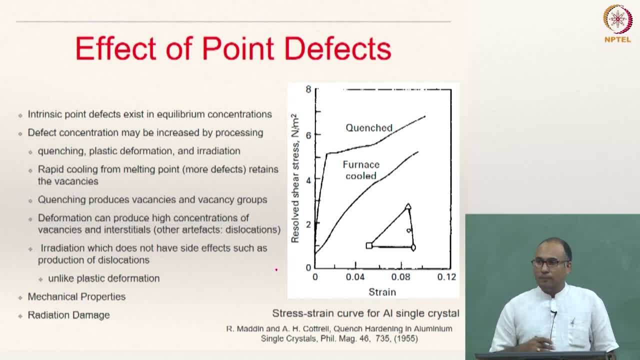 right, this is equilibrium concentration of vacancies. So the intrinsic point defects, they always exist in equilibrium concentrations in every real material. And this concentration of these defects, the concentration of this point defects, can be increased by different kinds of processing. You can actually increase the point defects. 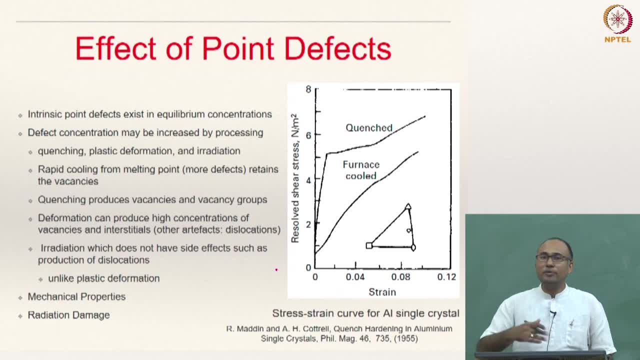 in the previous class. So in the previous class there were some points defects, but by thermal activation or actually doing some mechanical work as well, right, So you can actually increase the concentration by quenching. quenching is not quenching. 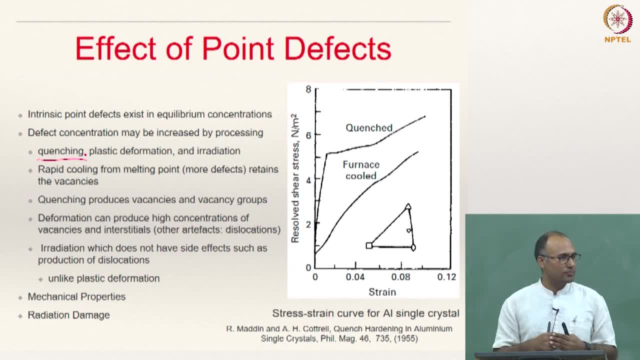 means sudden cooling of the material from high temperature. okay, And you can also do plastic deformation. by plastically deforming the material, you can increase the number of defects in the material. And another way that the point defects in particular can be induced in a material is: 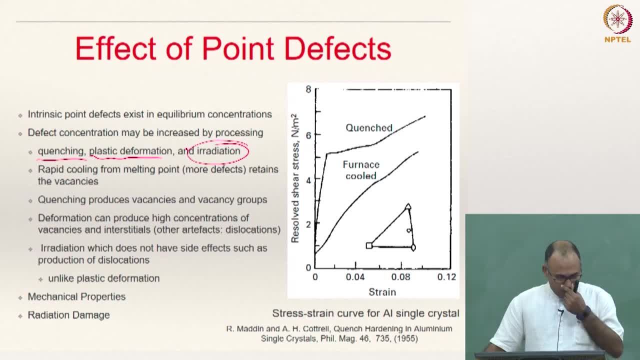 through irradiation okay. however, the irradiation is the nature of point defects that are generated due to irradiation. Irradiation is something that is that actually needs to be looked at, so we will discuss about the effect of irradiation on material in a moment. 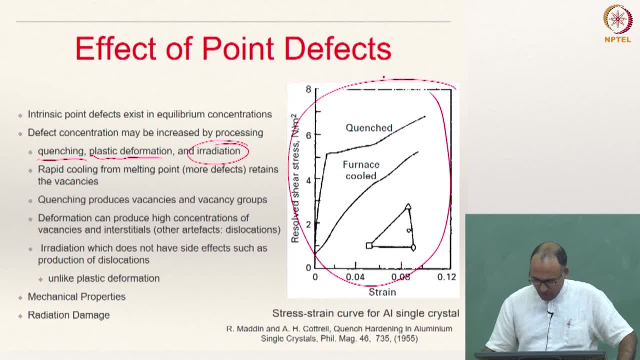 And if here, if you you see this graph, this actually shows the stress strain curve for aluminum single crystal, And there are two lines. one of them is a quenched sample, another one is a furnace cooled sample. Both these samples are irradiated. 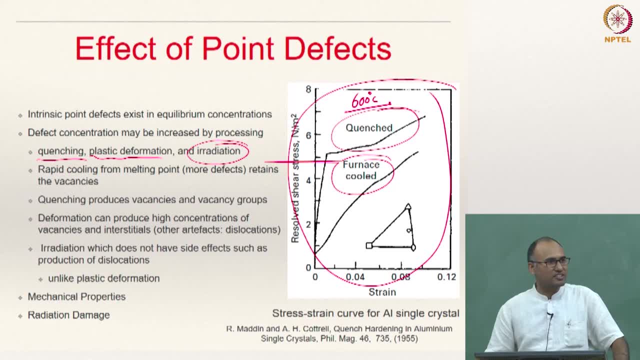 Okay, Both these samples are cooled from 600 degrees Celsius. they are initially at 600 degrees Celsius. this is an aluminum single crystal sample And one of them is quenched. that means suddenly cooled, maybe by putting in open air or in. 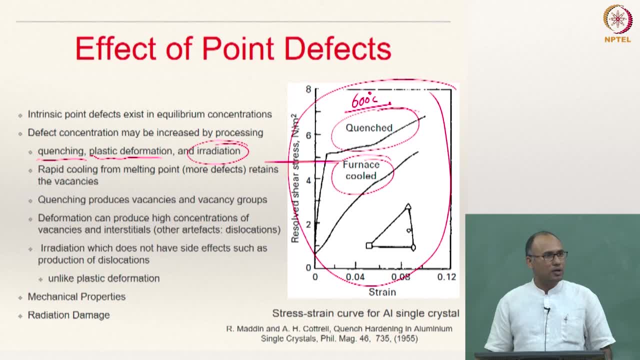 water. so the rate of cooling is very high And the other one is furnace cooled. that means you keep the sample in the furnace and gradually reduce the temperature of the furnace and hence it is much lower rate of cooling And you can see that, the mechanical behavior, and then you bring them to room temperature. 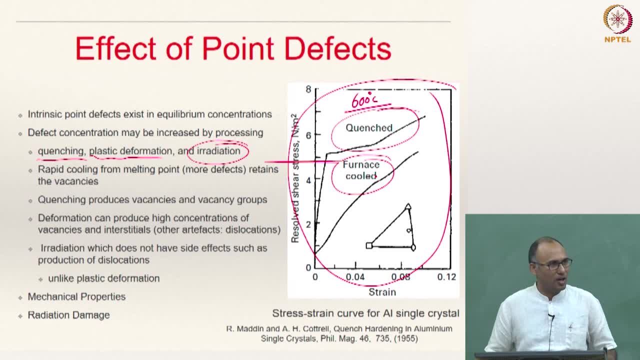 in both these cooling methods and then do the testing on this sample, And then what you would see is both of them behave differently. The quenched sample shows much higher strength compared to furnace cooled sample right. So that means what is happening is because of quenching. you are imparting point defects. 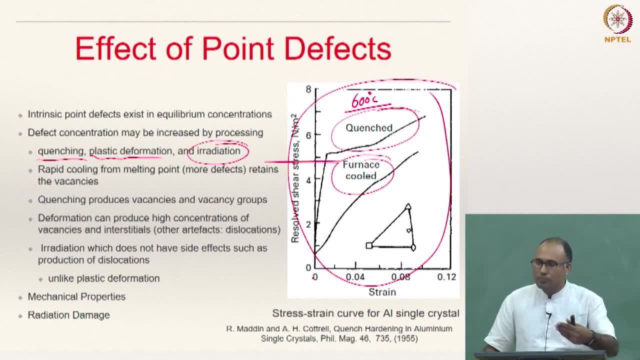 to the material, Or you are introducing defects in the material and these defects act as barriers for plastic deformation, And the rate of the number of defects that you produce depend on the rate of cooling. And that is why- because in quenching the rate of cooling is much higher and hence you. 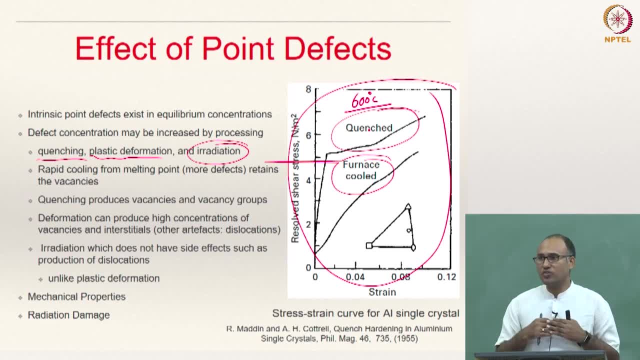 will produce more defects, and then you have more obstacles for plastic deformation, right. So if you actually quench a material, you are going to increase the strength of the material, right? The yield strength of the material is much higher here in this case compared to. 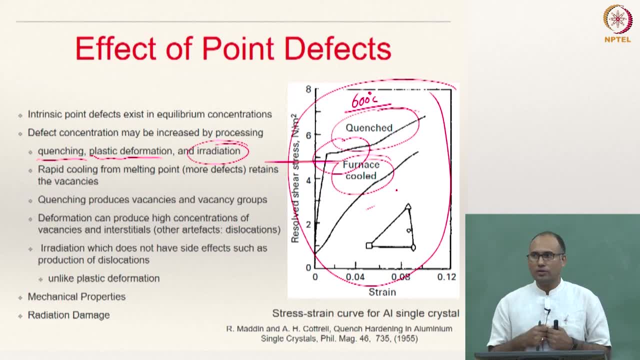 But then it also comes with a problem, right? You are reducing the ductility. That means the material becomes brittle, So you might increase the strength, but at the same time you are reducing the ductility or you are increasing the brittleness of the material, which may not be a desirable property. 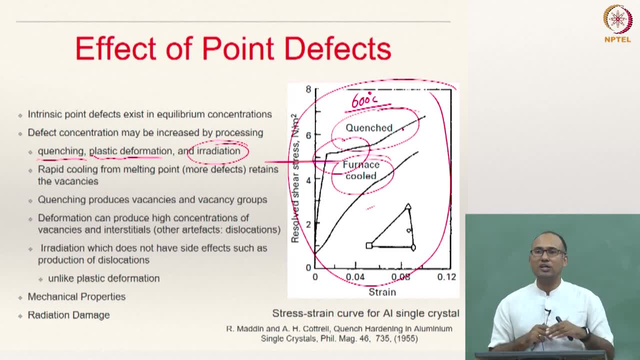 all the time. You might also want to increase the strength, but at the same time, you do not really want to sacrifice your ductility, You do not want to impart brittleness in the structure of the material Right. So you need to understand how the defects that are generated due to through different 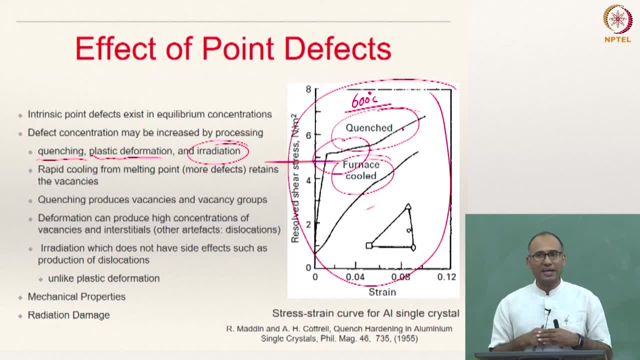 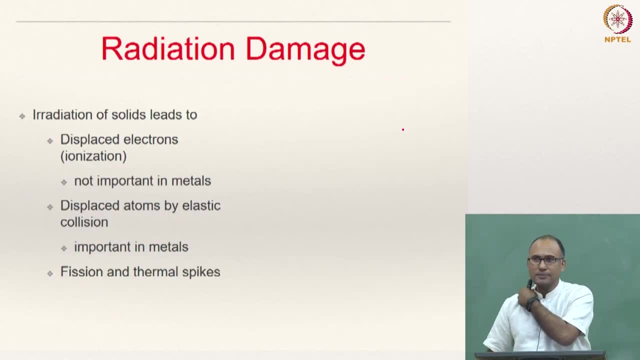 processing route contribute to the mechanical behavior of the material, right. So next now let us look at radiation damage. So what do we mean by radiation damage? When a material is subjected to radiation, the radiation can be. that means the radiation. 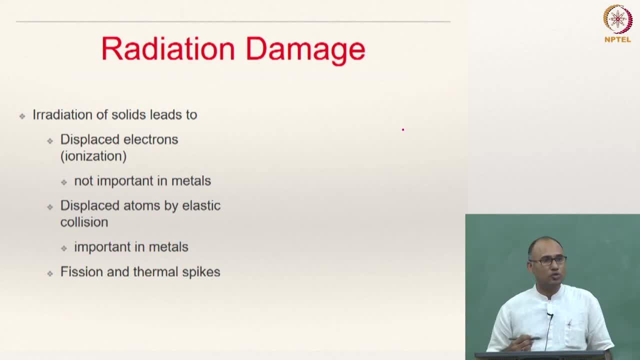 can be through different means. so you can have neutron irradiation, ion irradiation, right. So different particles going and hitting the material, right. So irradiation of solids in general can lead to different things. They can actually ionize the material. 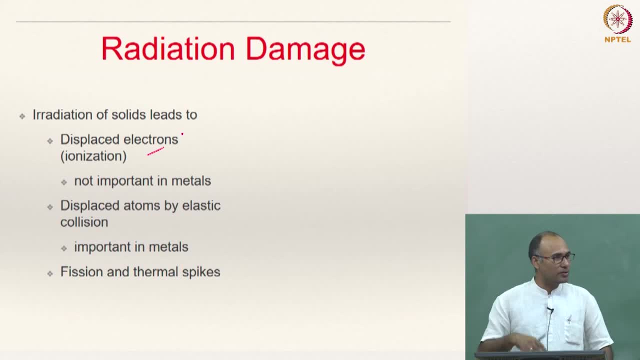 That means they can actually displace electrons. They can knock out electrons from the shells around the nucleus and hence ionize the material, which is not typically possible, Right? So this is the mechanism that you observe in metals particularly, or you can actually. 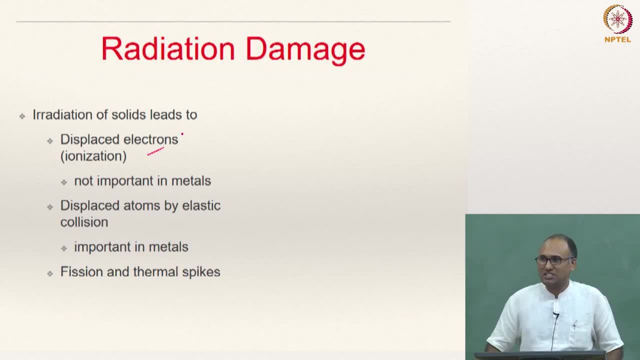 displace atoms from their lattice sites, Metronographic lattice site. the atoms will be sitting and you have, you impart, you subject this to irradiation and then, because of this irradiation, you can actually displace atoms from their lattice position. 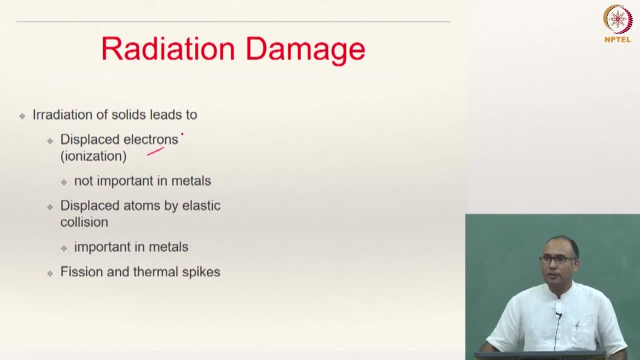 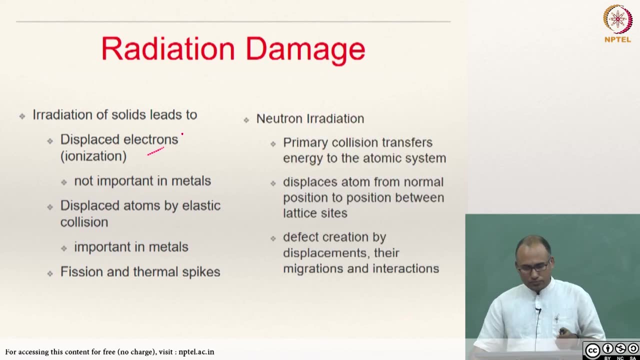 Right, This is one of the important things. So this is the mechanism that you observe, in metals particularly, And damage mechanism when a metal is subjected to radiation, Right? So let us look at neutron irradiation, which is typically the major problem that is observed. 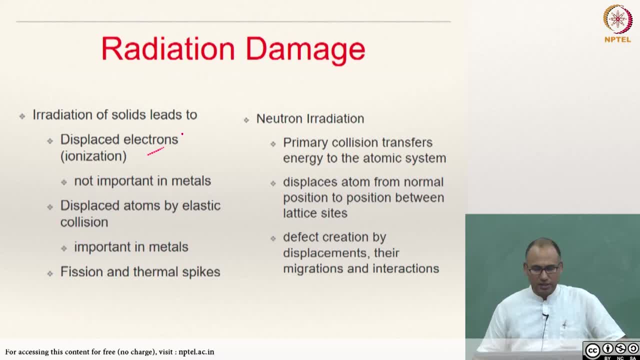 in nuclear reactors, Right, So you have high energy neutrons. These high energy neutrons, high energy particles, go and hit the structural material. So we have a nuclear reactor, Right, It is made of some special steel, The shell is made of some kind of special steel, and then these high energy neutrons. 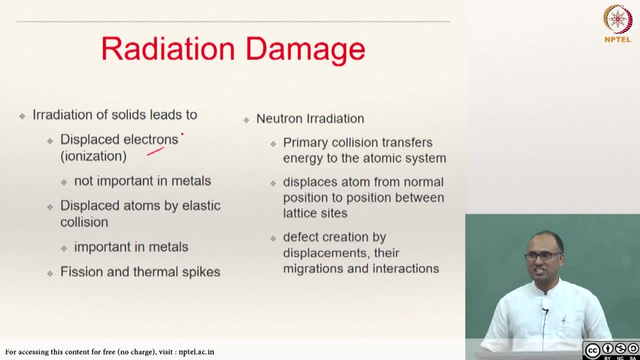 go and hit the surrounding casing material right And because of that they can actually displace atoms from their crystallographic lattice position. And when you have a very high energy neutron coming and hitting an atom and the atom displaces, then what happens? 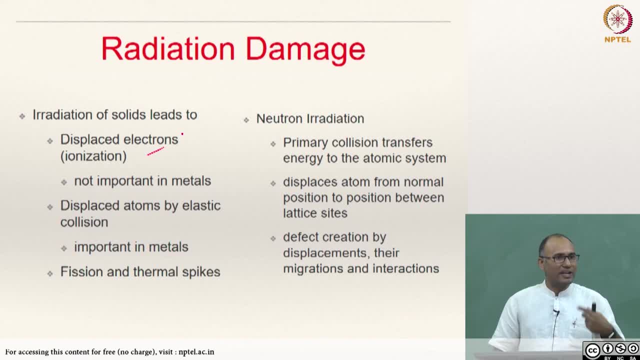 You are having a break in. you are actually creating point effect. So imagine you have a crystal right. So imagine you have a crystal, nicely ordered crystal like that. Crystal means you have this order in long range. And let us say you have a high energy neutron coming and hitting this guy. if the energy 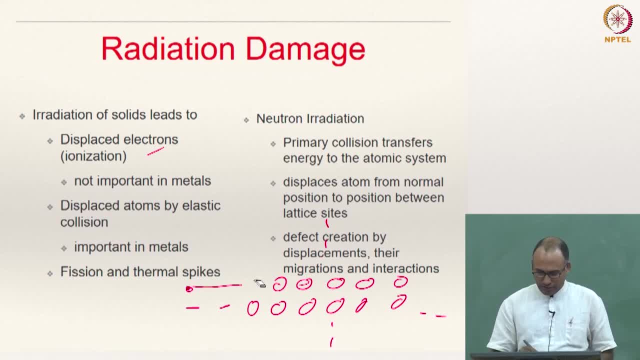 is sufficiently large, Then what happens? This guy will be knocked off and it may be going and standing there or elsewhere. It may be moving to some other position in the crystal lattice because of the high energy that you have imported. So you have created a vacancy. 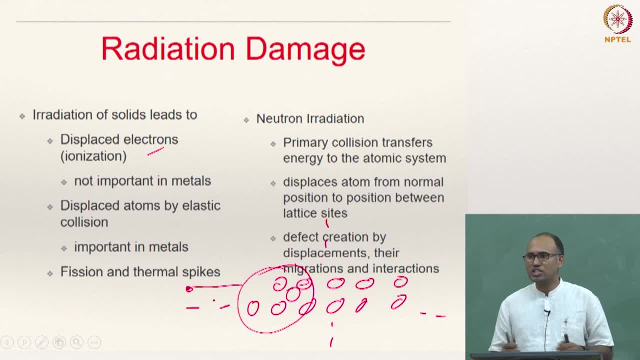 And locally. what happened? Locally the order got disturbed. So if you actually try to see, look for the order, crystalline order, then your local order is disturbed Locally. it is not crystalline anymore. Why? But if you have so many such high energy neutrons they can be bombarding everywhere in your 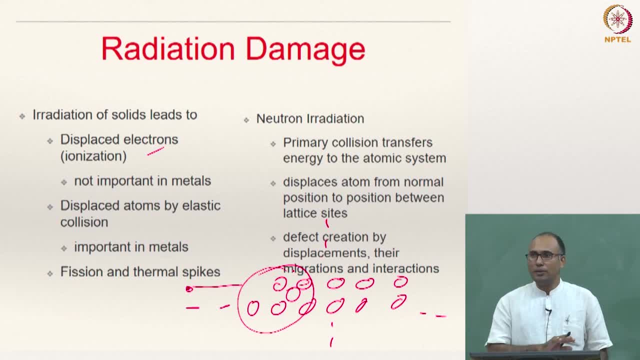 material and in the long run they can actually make your material non-crystalline. You can actually get your material amorphous right, So you create so many point defects. So the primary collision that means when a first neutron comes and hits an atom, the 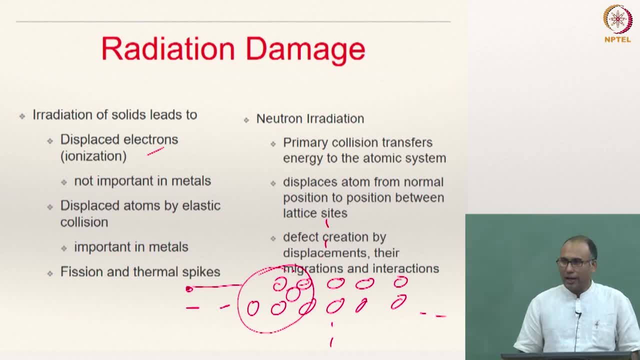 energy will be transferred to the atomic system And usually you will displace the atom from its normal position to somewhere in between the lattice side. It can go anywhere because it has high energy. It can actually stretch the bonds and actually fit in the interstitials. although the space 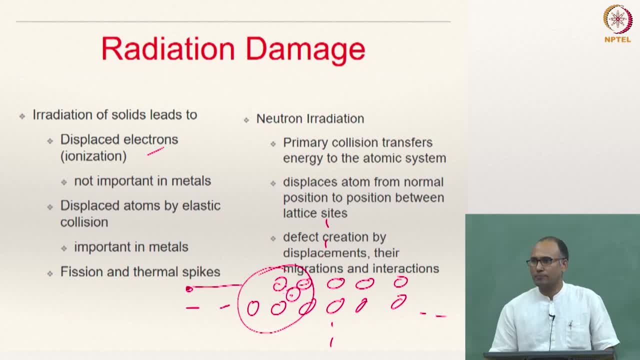 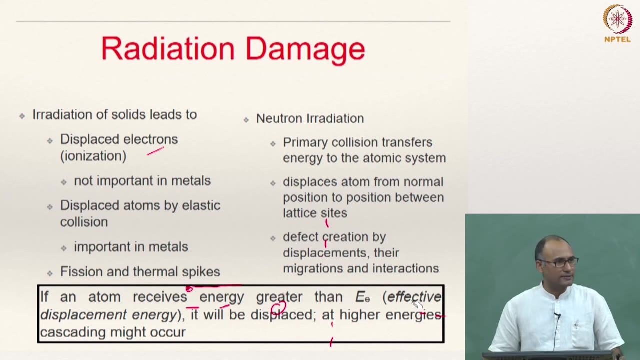 is not enough. But now it has energy, it can push aside right, And thus you create point defects in the case of radiation. So if an atom receives energy which is greater than effective displacement Right, Effective displacement energy, What do you mean by this effective displacement energy? 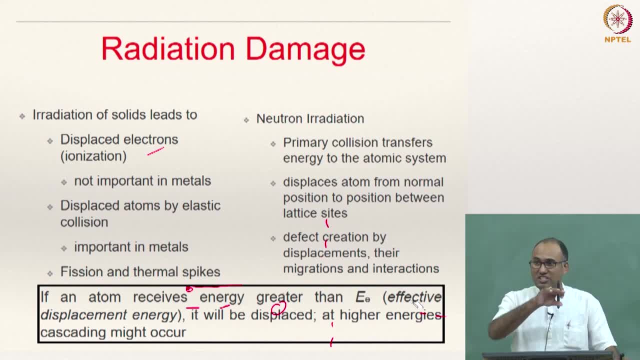 Energy that is required to displace an atom from its equilibrium lattice position Right. If the energy supplied to the atom is larger than the energy required to displace the atom, then the atom will displace. Otherwise, what happens? Whatever energy is imported to the atom will be transferred to neighboring atom. 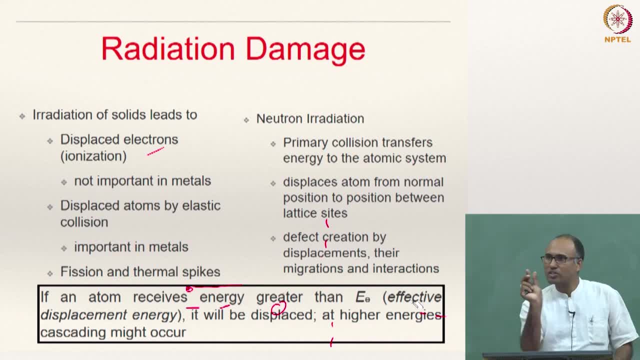 So the oscillation, the atom will be oscillating about the same distance. Right, It will be oscillating about its mean position and if you are giving a higher energy, then it will. its oscillation amplitude will increase and the energy will be transferred because 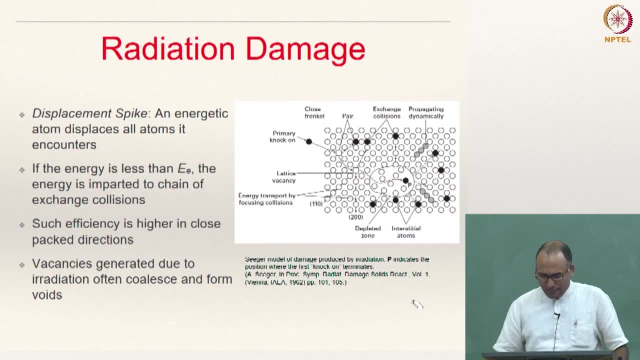 it is an elastic energy Right. So this is a typical picture of radiation damage, a cartoon that shows the various processes that one can discuss in the case of radiation damage, Right. For instance, if you have a high energy atom, if you add energy from a neutron very high, 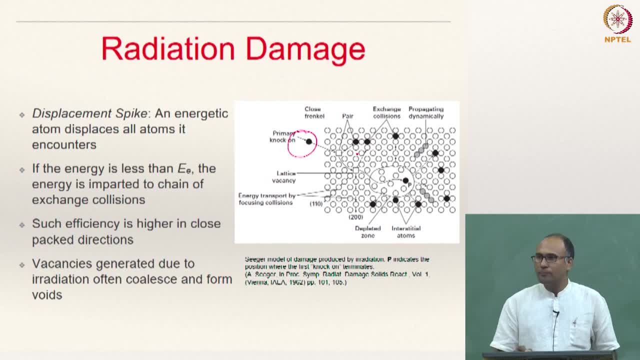 energy, neutron, for instance, this primary noxon atom. it will go and hit the atom positions in the lattice and then gradually they displace atoms from their actual position and create different kinds of big point defects. For instance, here you have a vacancy and here you have vacancy, interstitial pair and 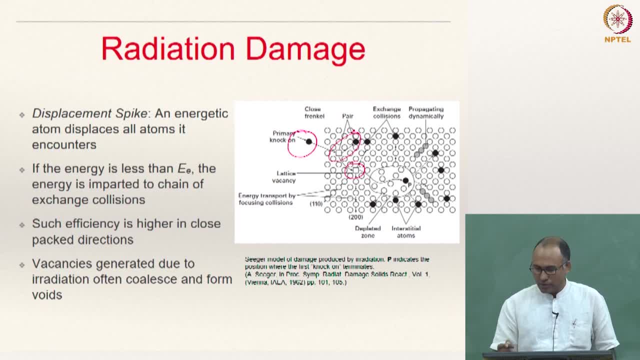 so on. Right And here, exchange collisions, and then here you have a large sort of void. Right And here you have created an interstitial atom, and so on. So this process of displacing an atom, an energetic atom, displacing all other atoms, 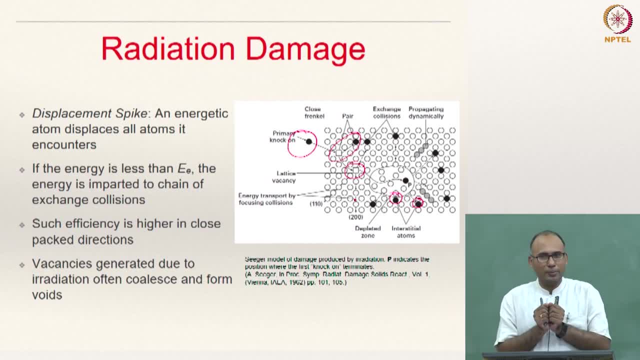 that it encounters in its path. so you have got some energy to this atom, and when this atom is moving, and whoever comes in its way, it actually pushes away and then gives away energy to this Right To the surrounding atom. Now this process is what is called displacement spike. 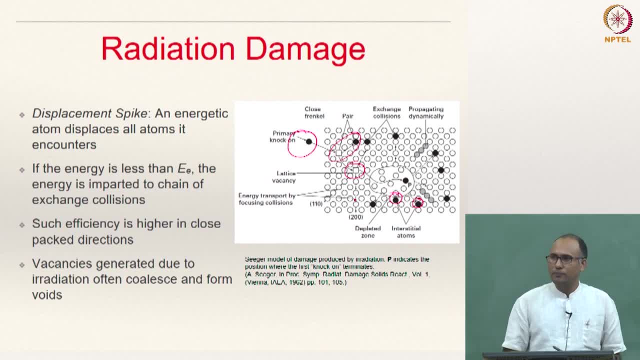 Right, And when this energy that is imparted to the atom is sufficiently large, and if it is larger than displacement energy E, then you will actually create point defects. And then these point defects are there, either vacancies or interstitial. They now act as obstacles to deformation, obstacles to plastic deformation. 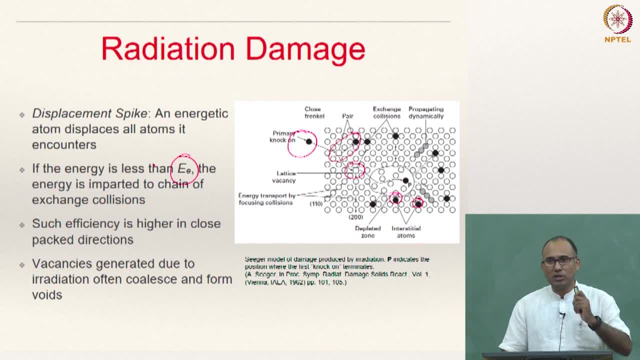 What do we mean by plastic deformation? We will see in a moment. So they actually act as obstacles. So if you create more and more point defects, all these point defects are going to stop the plastic deformation And, as a result, what happens? 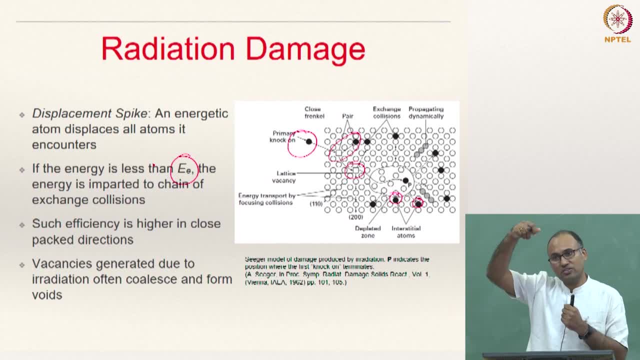 The material offers more and more resistance Right. The material offers more and more resistance for the deformation and hence you have higher yield strength. You will not be able to impart plastic deformation at a position where you would normally impart, when the defects are not present in the material. 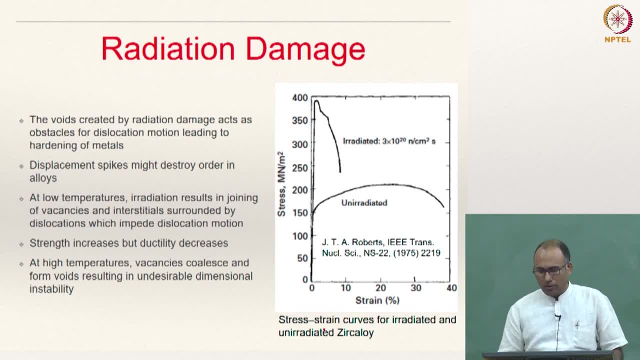 Okay, So this is again the stress-strain graph for zirconium alloy, zircaloy. This is an irradiated sample and this is an unirradiated sample. So this is the deformation, So this is the dosage. 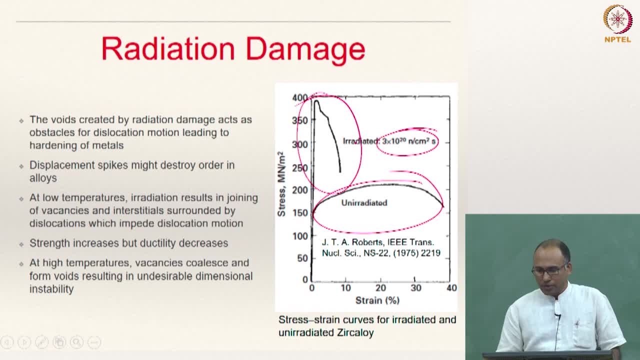 Right And you can clearly see that the material has become extremely brittle After this much of irradiation. the material has become extremely brittle. So if you take the area under this curve, compared to this guy, this area is much less. 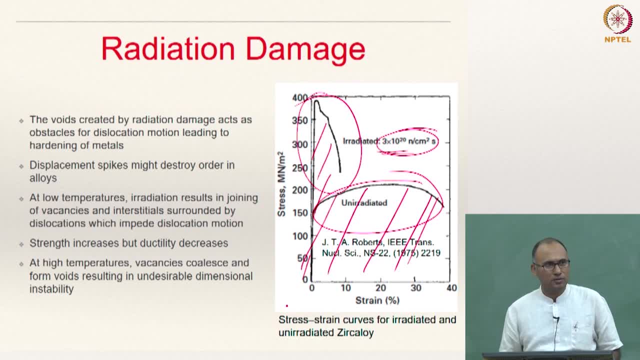 So what is this area? This is the energy of the material, This is the energy of the material, This is the energy of the material, This is the energy. So let us say this is fracturing here, This is fracturing here. 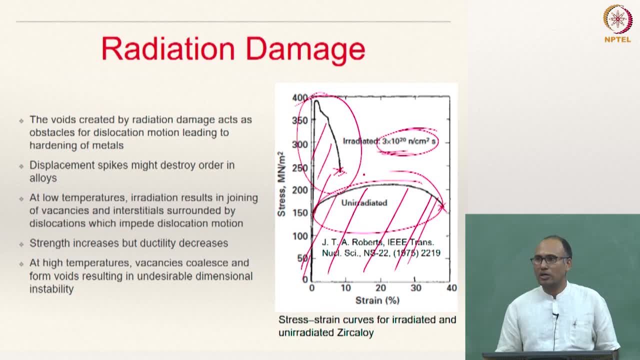 The total energy that can be absorbed by this material before it can fracture. Right Here you have much less energy and hence and also much less strain. Right Here you can actually go up to 35 percent strain. Here your strain is only 10 percent. 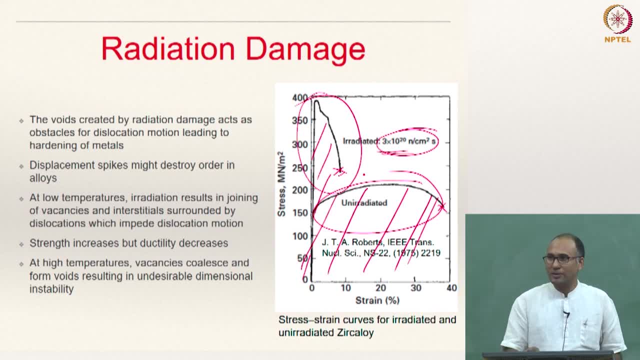 That means you are. you will not when the material breaks. you will not have a lot of energy, Right? So this is the energy. You will not when the material breaks. you will not have enough time for response, You will not be given enough sufficient number of notices that it is actually going to give. 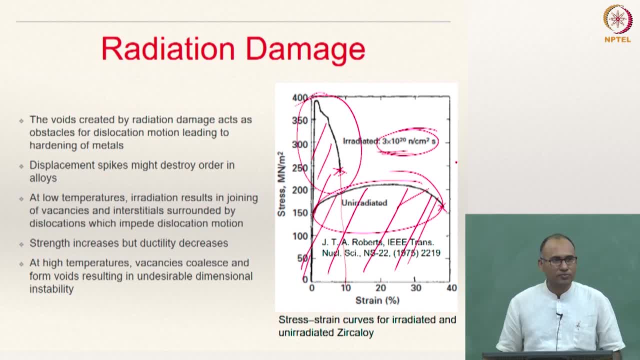 away, Whereas this material will give you some sort of an indication that this is going to break. And that is the problem with irradiation. You really do not want to have a material which gets embrittled during its service, And that is the reason why the design of pressure vessels that are used in nuclear reactors. 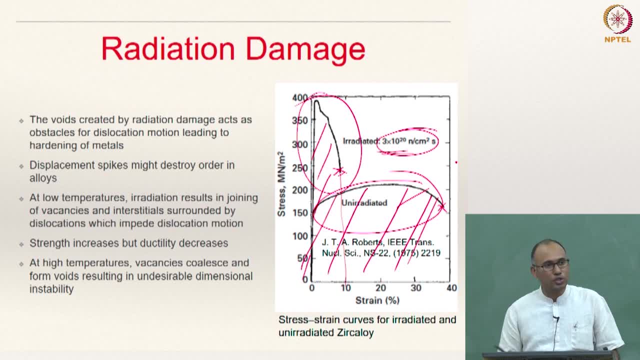 is an extremely important task, And one should do it carefully, taking into account of the effect of irradiation, And that is the reason why you need to check for the health of these materials from time to time, And otherwise they can create catastrophes. 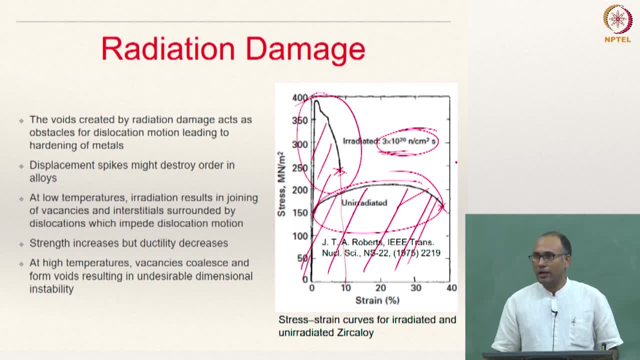 Because if your pressure vessel becomes brittle over time and even if you have a small crack, the crack dips through suddenly, right when it becomes a critical crack. the crack dips through suddenly in a brittle material as compared to, in comparison to a ductile material. 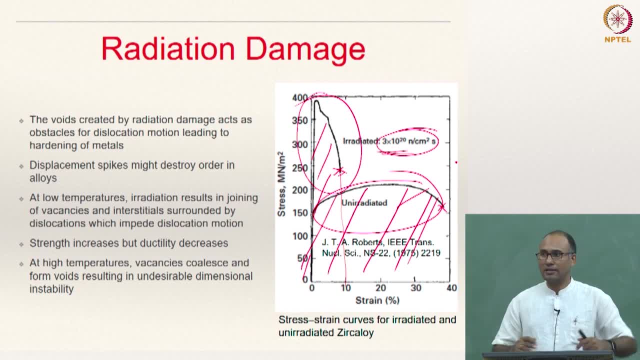 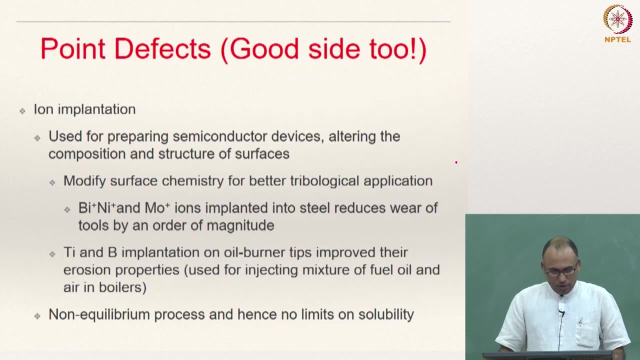 So you do not want to break this pressure vessel all of a sudden, because then it creates a much more dangerous accident. So that is the reason why you need to understand the effect of these defects on the mechanical behavior of these materials. So so far we have discussed these point defects and their how they affect the mechanical 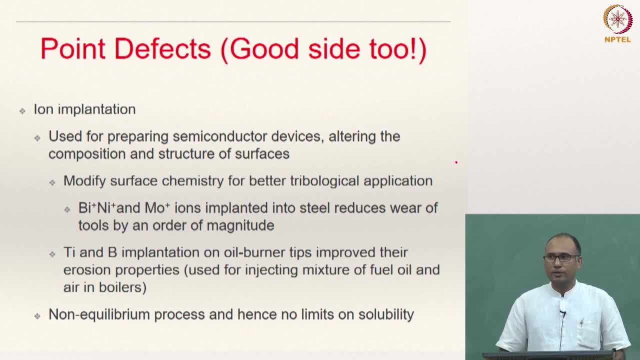 properties, how they are going to negatively impact the mechanical behavior of the material. But, as we have discussed, the defects are not necessarily always bad for you. sometimes they can also be good. For instance, the ionic material Right For ion implantation. you can use them for preparing semi-conductor devices and also. 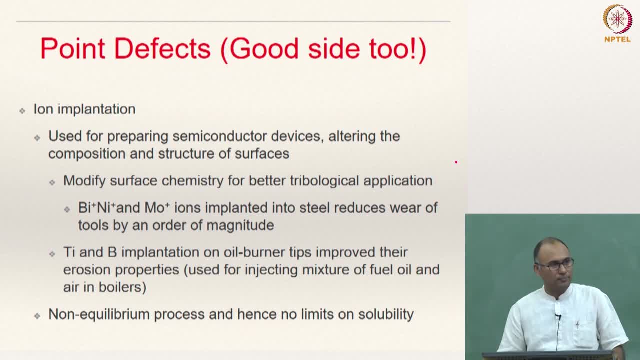 changing the composition and structure of surfaces of the materials Right. So for instance, for tribological applications. tribological application means where you have a lot of wear and tear right when two surfaces come in contact and then they are moving. 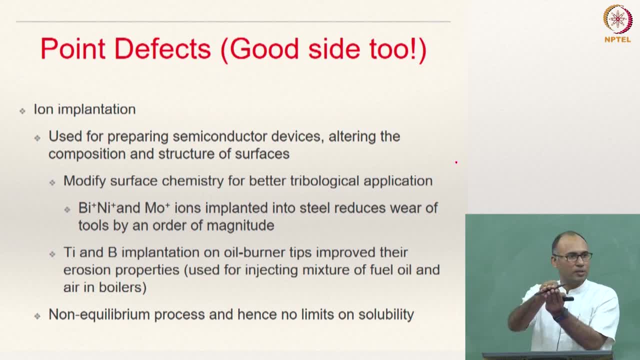 past one another, then you create there is a possibility for the material to get worn out over the time, Right? So if you have this wear, then you can actually do some processing to the surface, some surface treatment. So here you can actually people have shown that you can use this: bismuth, nickel, molybdenum. 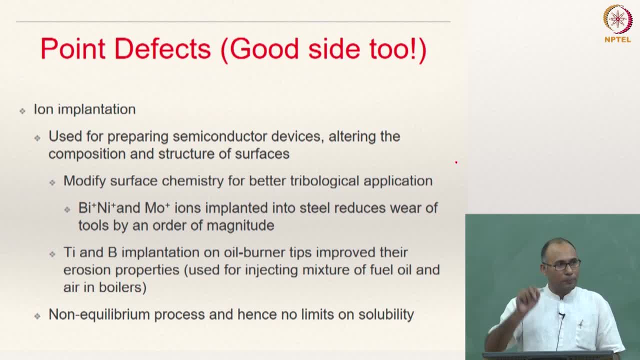 ions, and you can use them to implant on the surface of steel in order to enhance their wear resistance- Right. Similarly, titanium and boron implantation on oil burners- Right, Yes, Yes, Which is good, Because that improves their erosion properties, because they work at high temperatures and 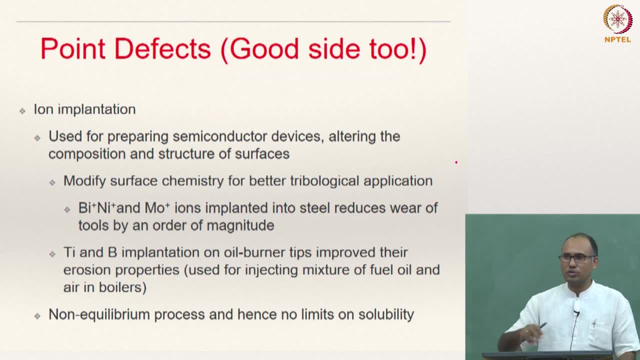 then you want to improve their erosion properties. So all that you need to do is you need to add, do some surface treatment. So basically, here they. if you do the ion implantation of titanium and boron, then that enhances the erosion properties. 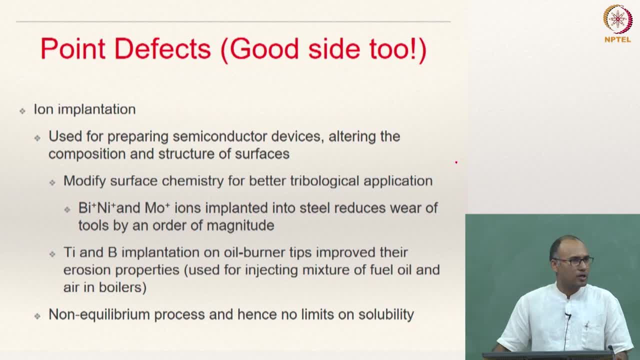 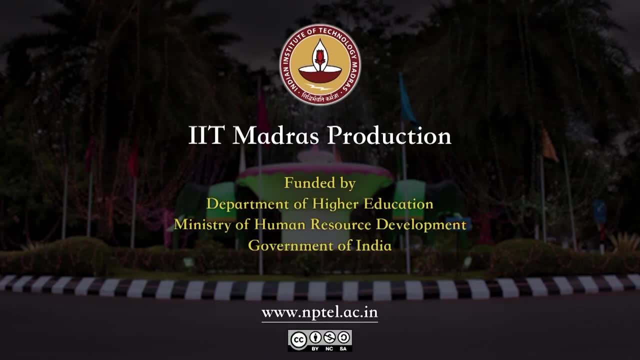 So you can like this. you can actually see several other usages. useful sides of point defects: Yes, Yes, you.